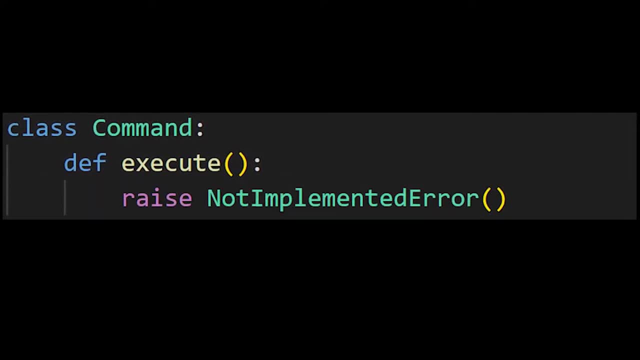 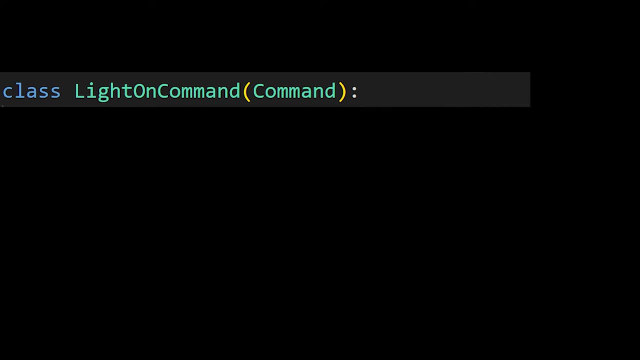 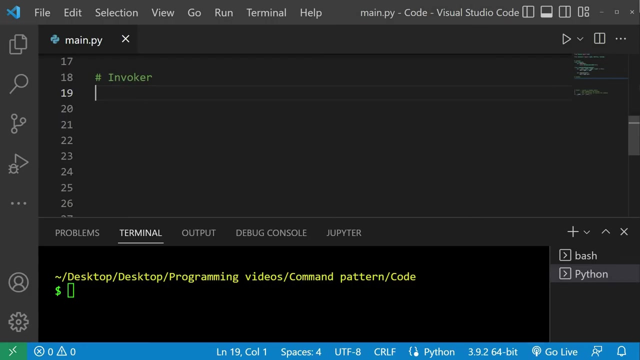 the interface will be just a class whose execute method will throw a not implemented error. Then let's create a single command for now, A lightOnCommand class, which will implement the command interface, whose constructor will take in a light receiver and whose execute method will call the on method on that receiver. Now let's define the remote class a bit differently. 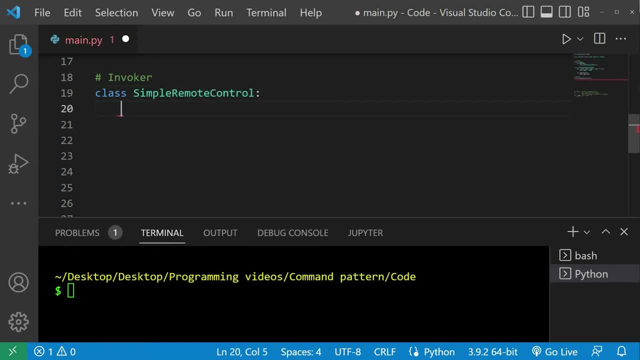 We'll call it a simple remote control and use it just to show what we are doing without too much noise. We'll redefine it to be a fully functional remote control in just a bit. The simple remote control class will have a single slot filled of command type. It will. 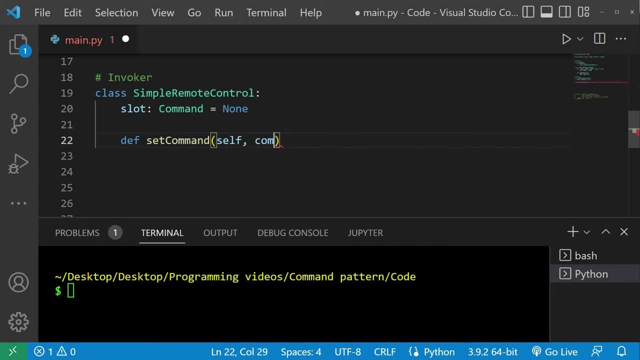 have a setCommand method that takes in a command instance and just sets the slot on the remote to the passed-in command. It will also have a buttonWasPressed method that will call the execute method on the stored command instance. Now if we create an instance of the simple 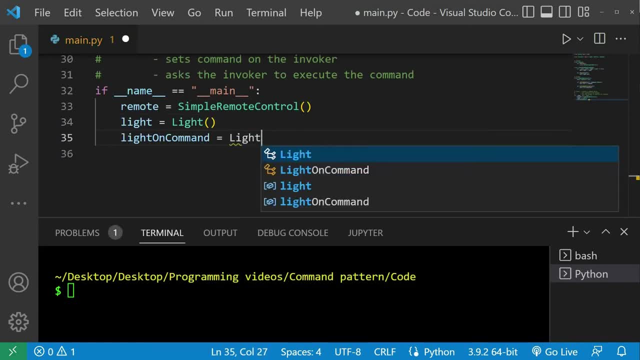 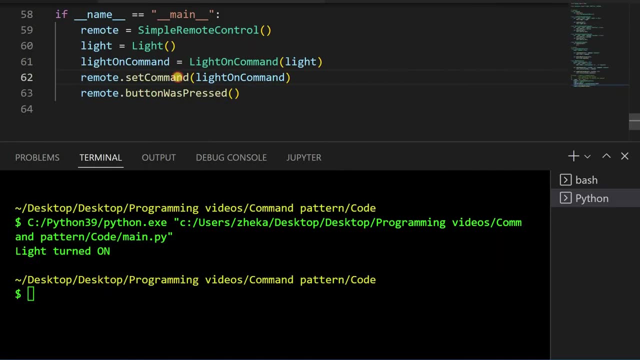 remote control, set the lightOnCommand on the remote and call the buttonWasPressed method. we see that our simple remote is now functional. Before we go to implement the fully functional remote, let's see what happens if we call buttonWasPressed before setting the command. 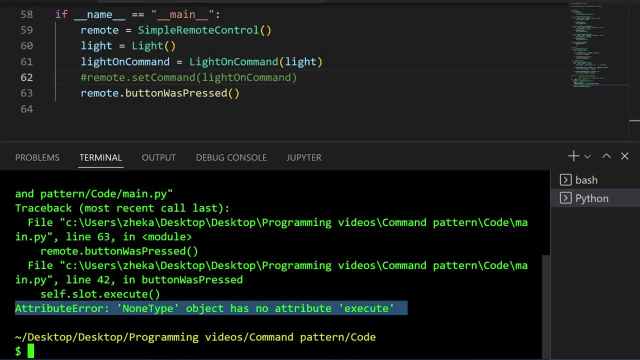 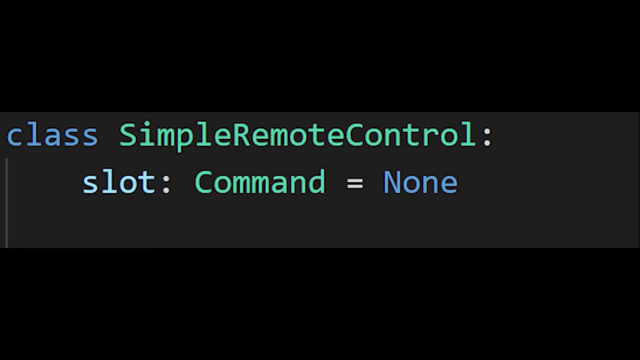 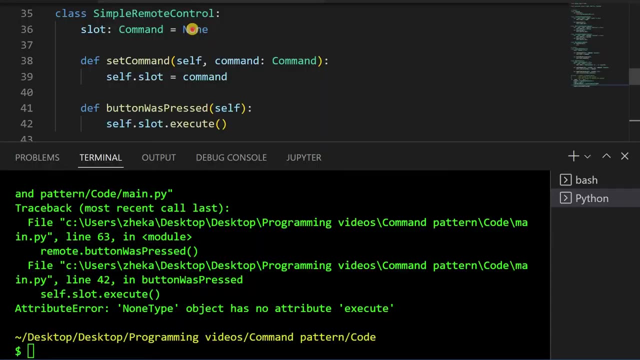 error: NoneTypeObject has no attribute error. NoneTypeObject has no attribute error. That's because we set the slot field to not by default. What we can do instead is define a new command. We can call it noCommand, Which just does what I do most of the time: Nothing. Now we can set. 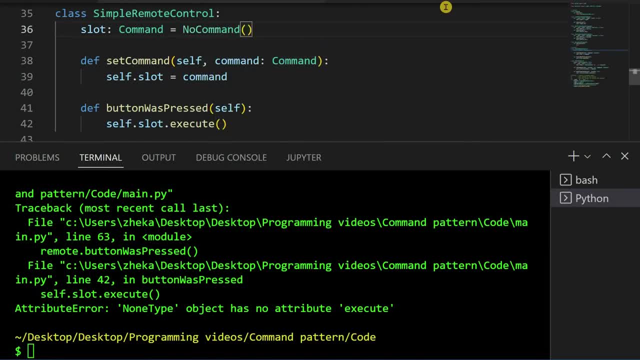 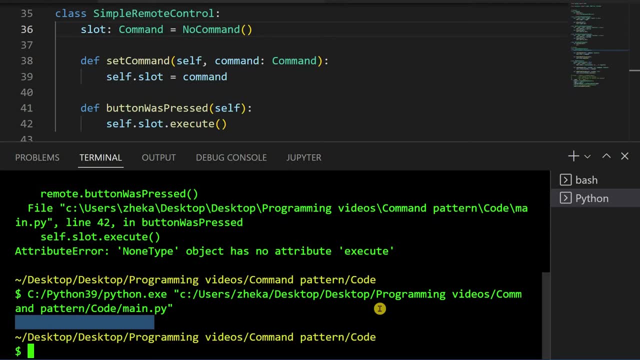 the slot field to an instance of noCommand instead, and our remote won't do anything but also won't give us errors. Before we go and rewrite our remote again, let's look at the command pattern diagram. There are four components. We've already seen. 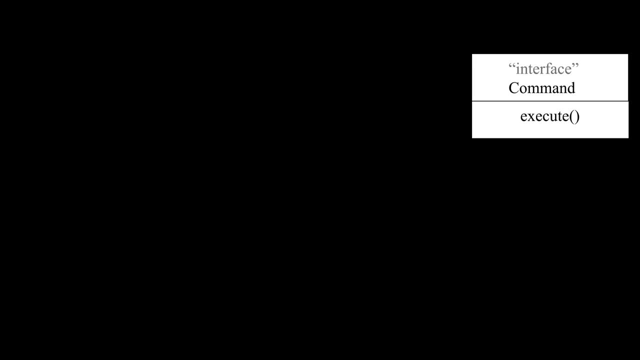 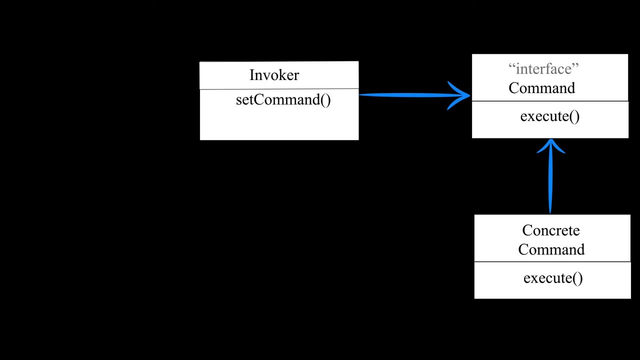 the command interface. Typically it will have a single method execute on it. They invoke or. sender is the remote control class. All it does is store a reference to a command or multiple commands and send a request to a receiver. The receiver is the class that contains the actual. 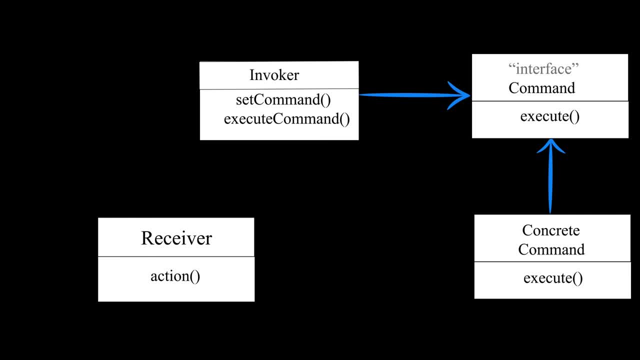 business logic. So in our case, light is the receiver. Finally, we have the client. The client creates the command object and configures the remote. The client, in our case, is our program. after the if double underscore name: double underscore double equals double underscore main.